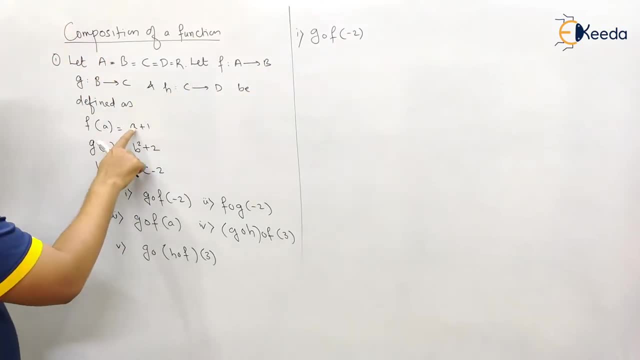 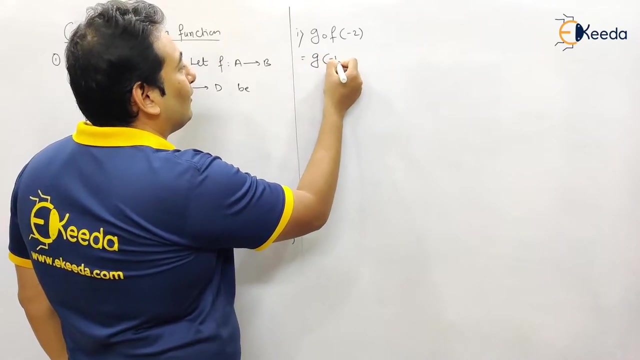 minus two. so what is f of a? f of a is a plus one. if you want f of minus two in place of a, if you put minus two, so this will be minus two plus one. so minus two plus one will be minus one. so that is g of minus one. 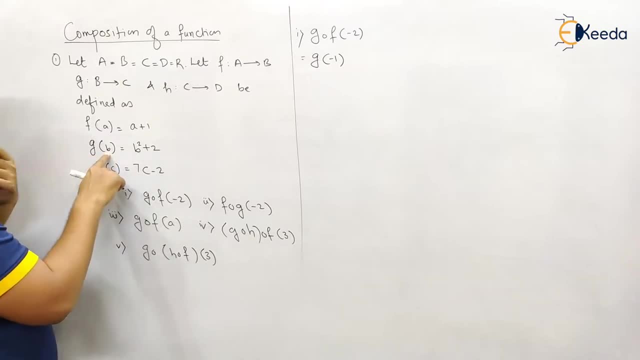 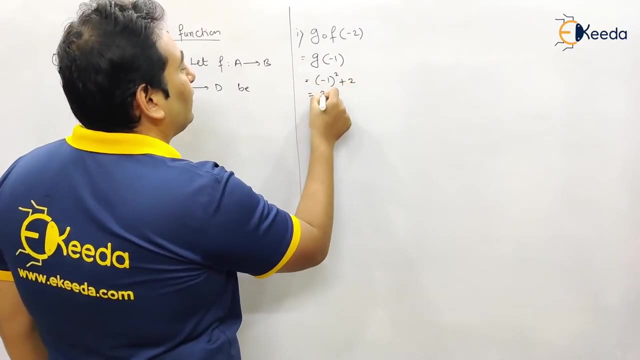 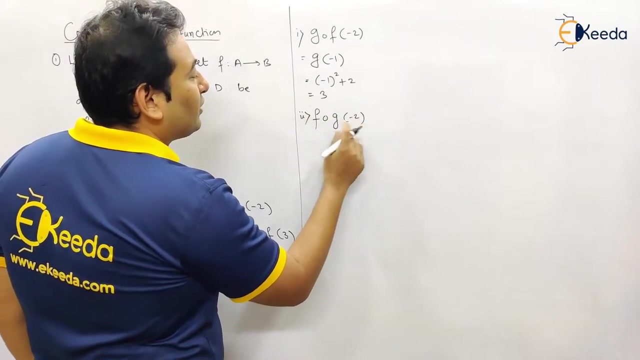 g of minus one. that means, in place of b i'm going to put minus one, so this will be minus one square plus two. that is three done. done with the first problem. let us start with the next problem: f of g of minus two. so first of all, g of minus 2. we're going to find it out. 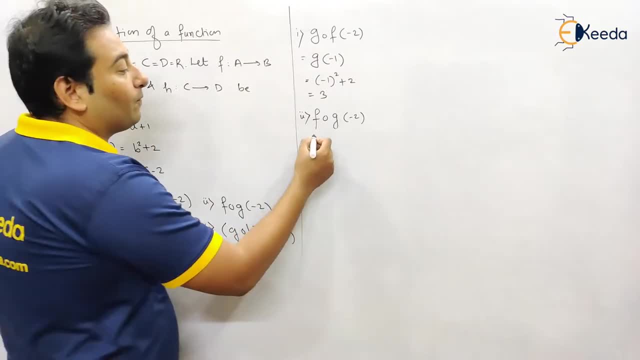 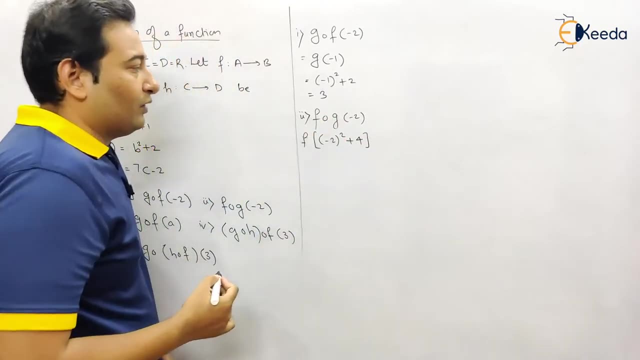 in place of b minus 2, so that is minus 2 square plus 4 g of minus 2, so that is 4 plus 4 g of minus 2, so that is 4 plus 4 square plus 4 g of minus 2, so that is 4 plus 4 square plus 4. 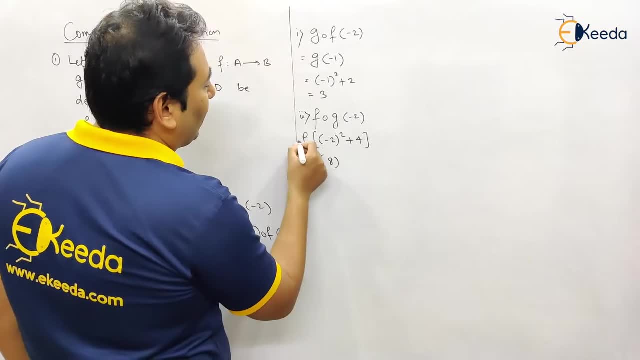 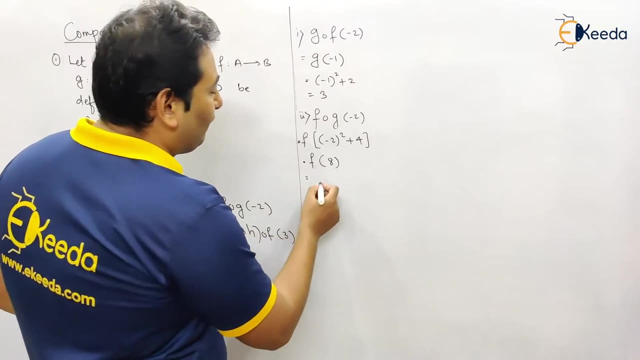 So that is 4 plus 4 is 8.. So we need to find it out: f of 8., f of 8.. So in place of a we have 8.. So 8 plus 1 will be 9.. 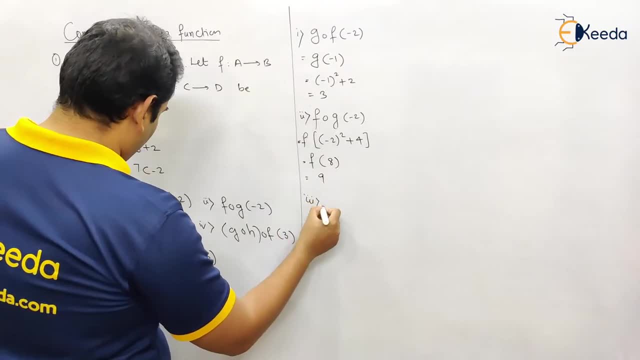 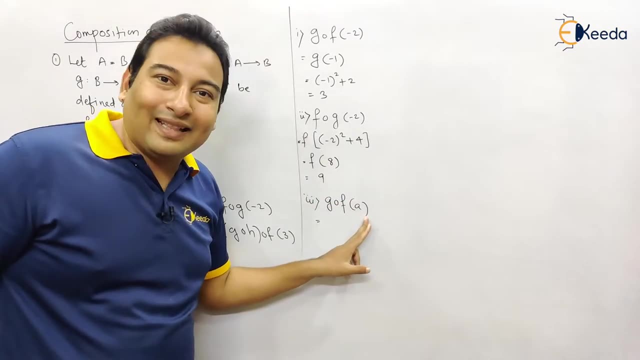 Let us start with the next example, number 3.. g of f of a. Here it is f of a. That means, in place of a we're going to keep a only. So f of a is a plus 1.. 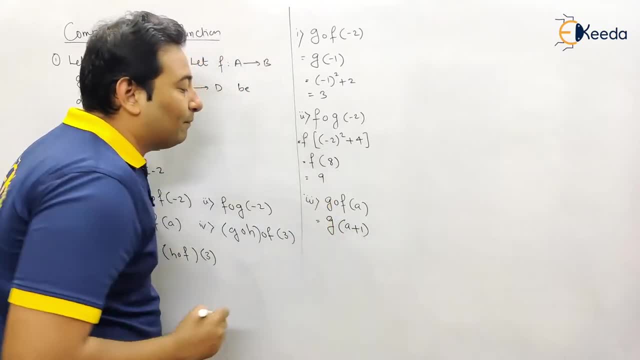 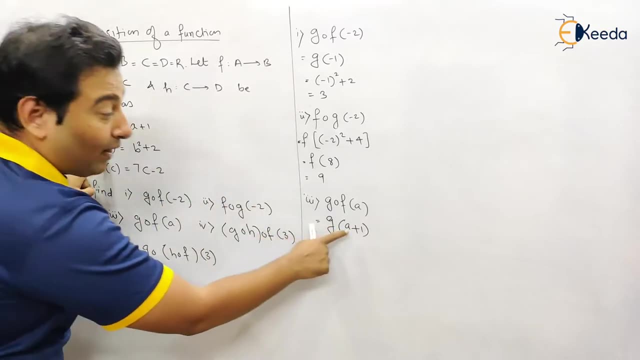 So in short, it will be g of a plus 1.. Because f of a is a plus 1 only. Next is g of b. So in place of b now I'm going to put a plus 1.. So this will become a plus 1.. 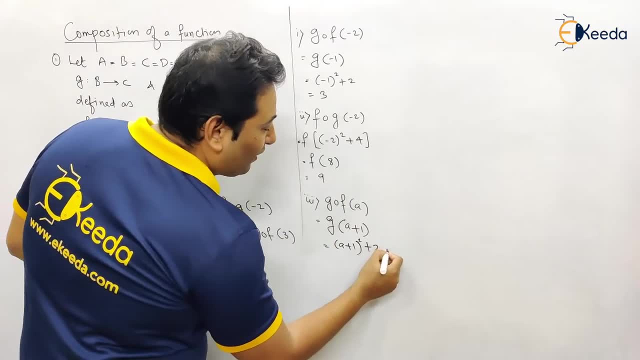 In place of b, a plus 1.. So a plus 1, the whole is square. This plus 2 will remain as it is. Next number 4.. Now, if you observe number 4 and number 5, see here. 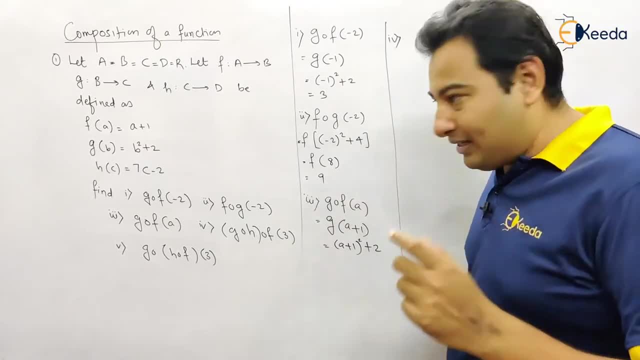 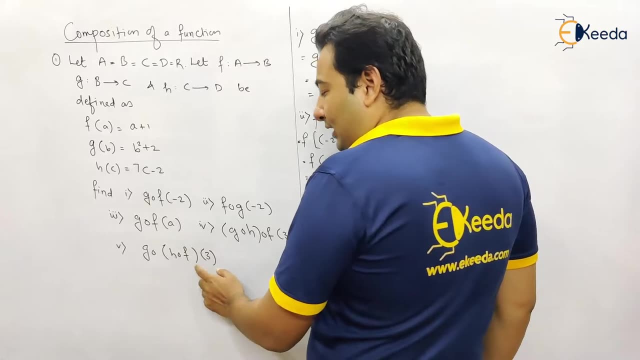 As I told you, this brackets and overrides O, doesn't matter. So if you see the order, first of all f of 3 will be evaluated, Then h and then g. Here also the same order: f, h and g. 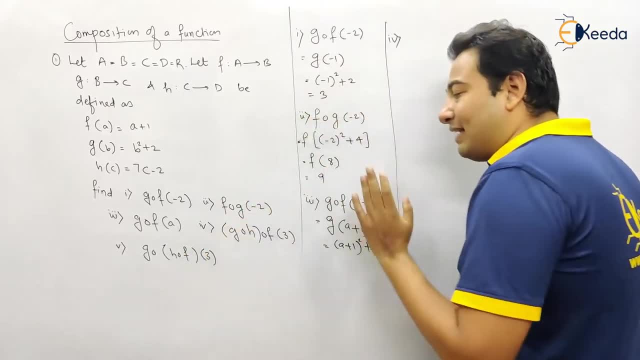 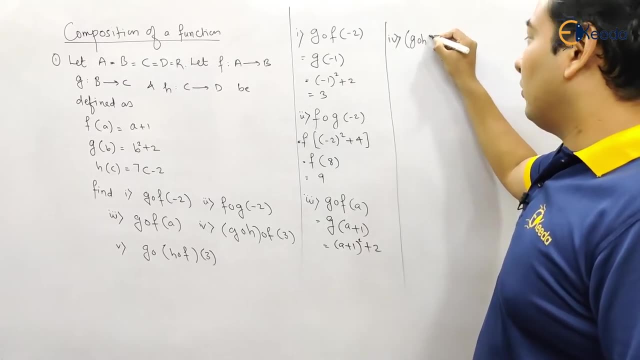 So, in short, both the problems are same And both will give you the same result. The brackets o doesn't matter, So let us evaluate first g of h, of f, of 3.. First of all, f of 3 will be evaluated.